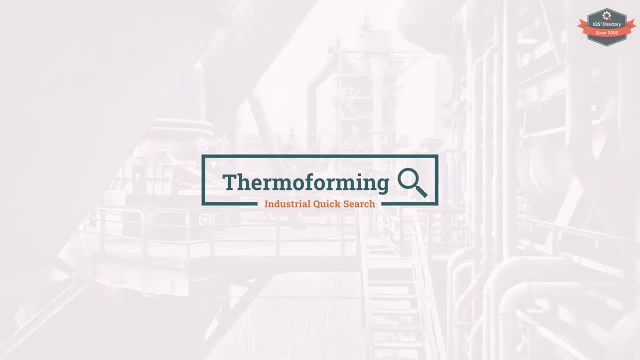 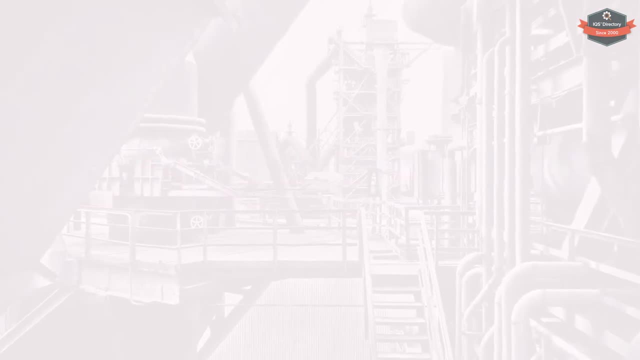 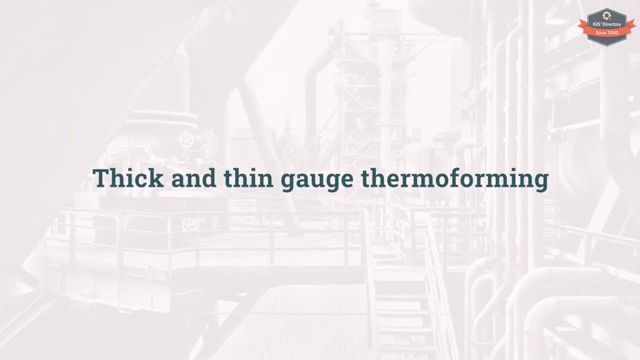 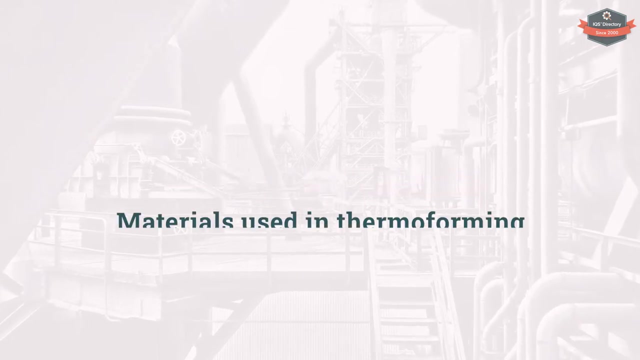 This video presents all the information you need to know about thermoforming. Topics discussed are the following: What is thermoforming? Thick and thin gauge thermoforming, The thermoforming process, Types of molds, Thermoforming methods, Materials used in thermoforming. Problems and quality issues encountered during thermoforming. 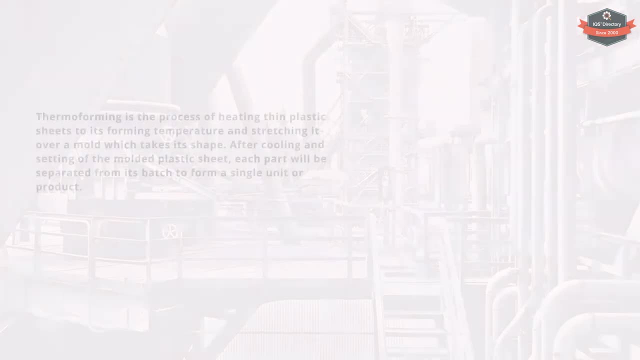 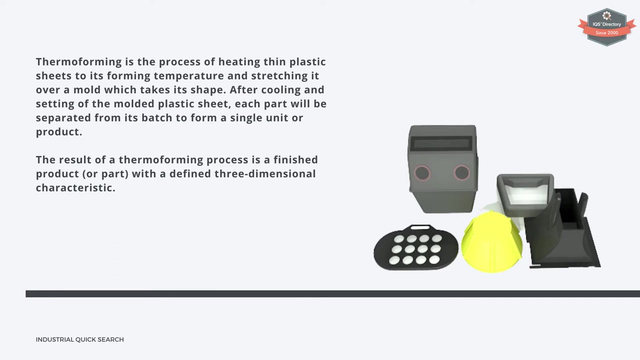 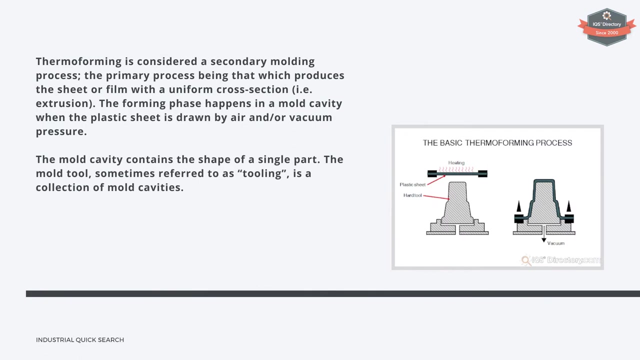 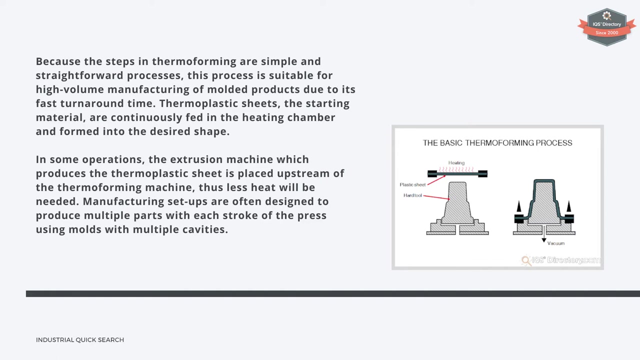 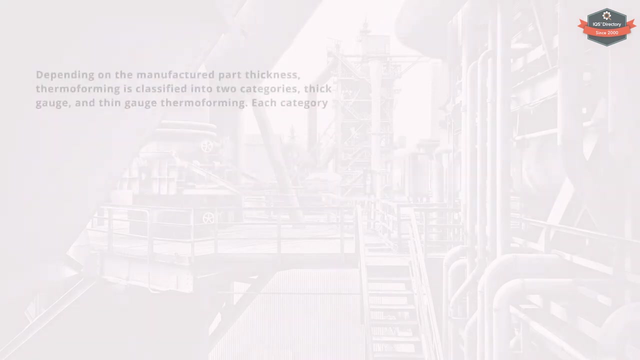 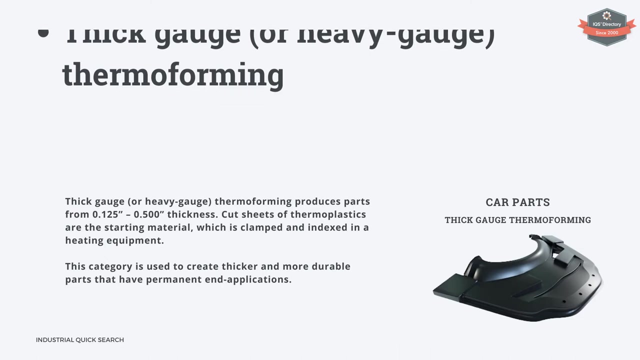 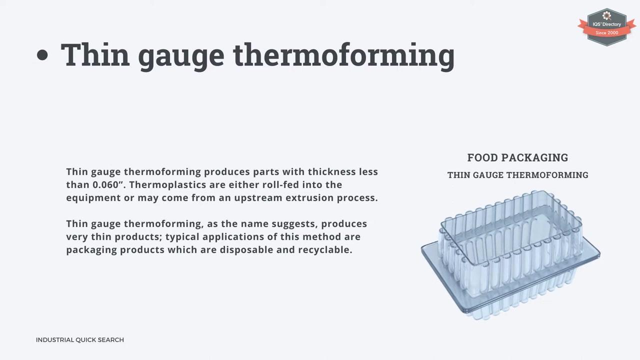 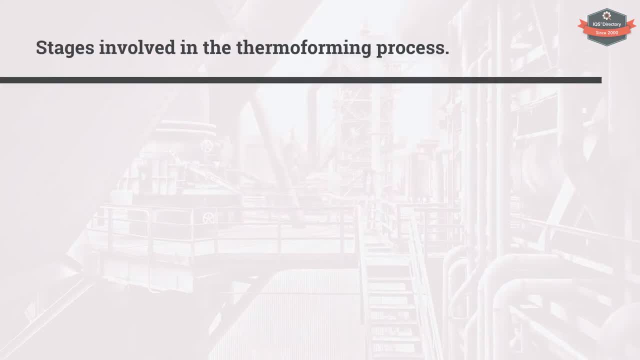 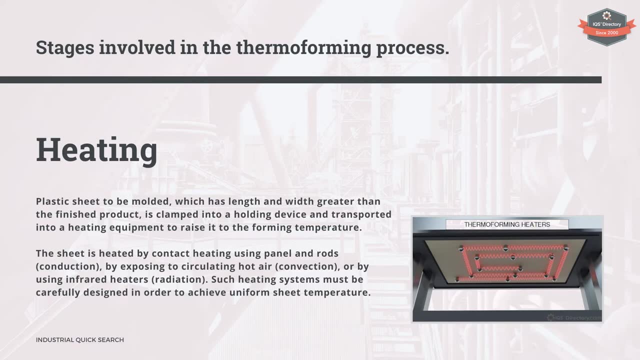 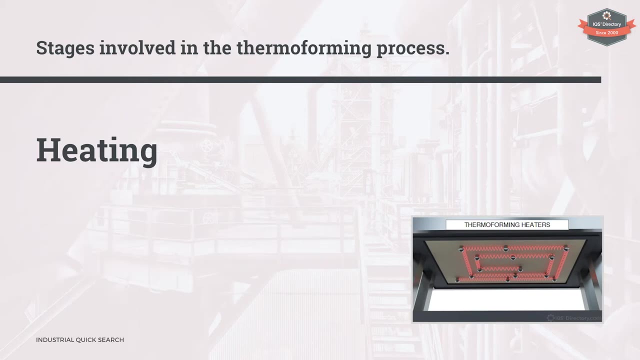 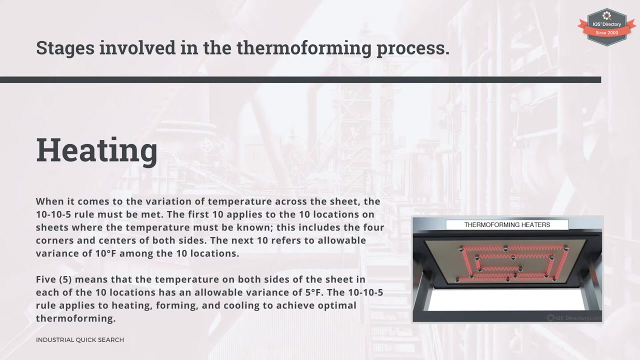 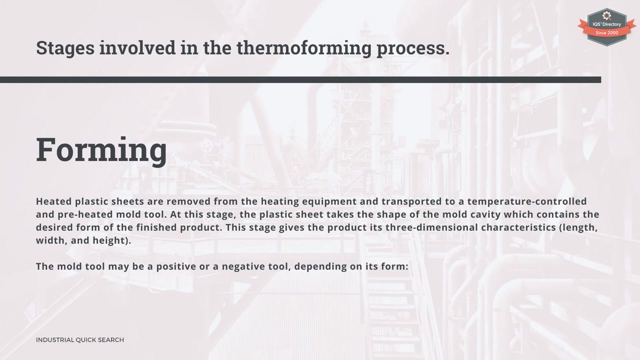 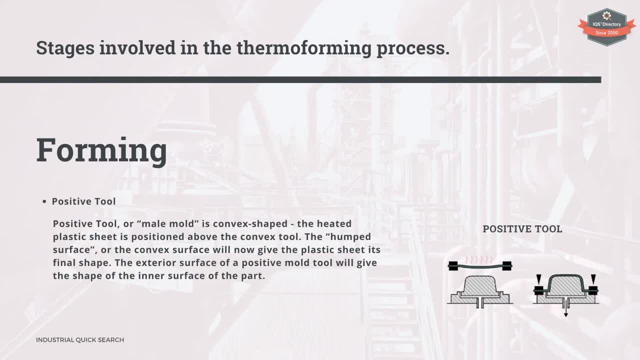 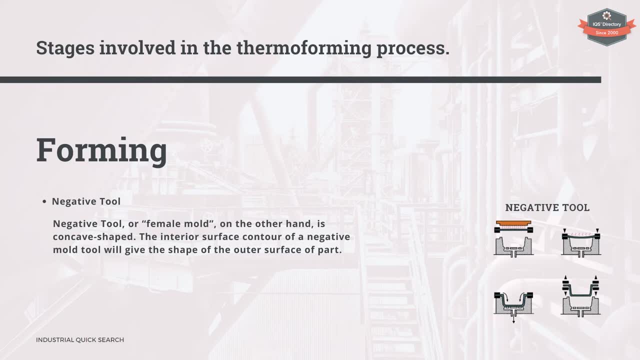 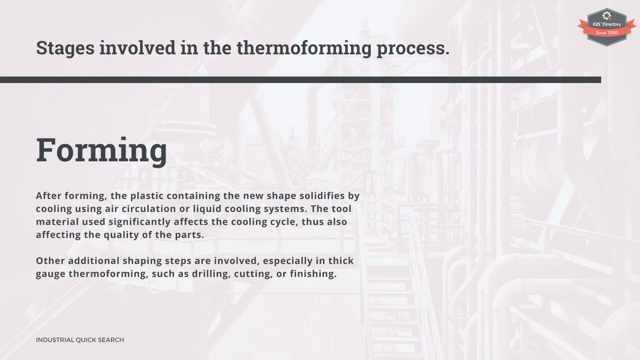 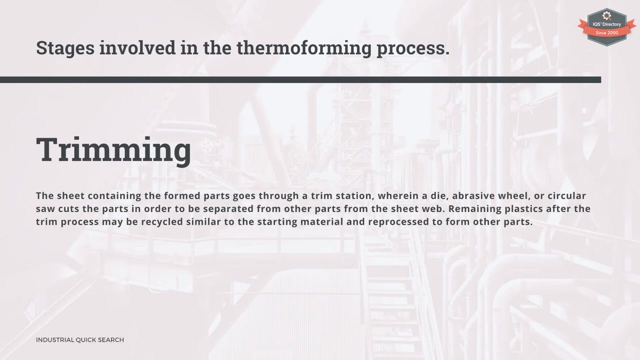 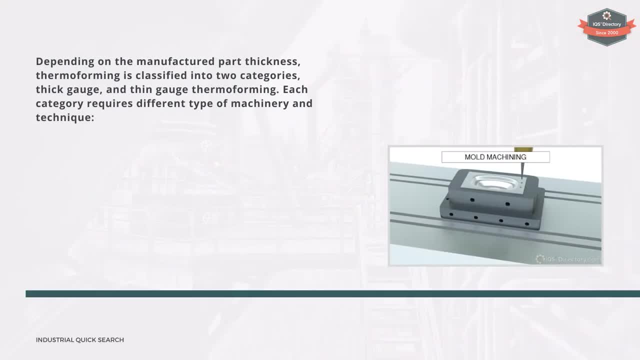 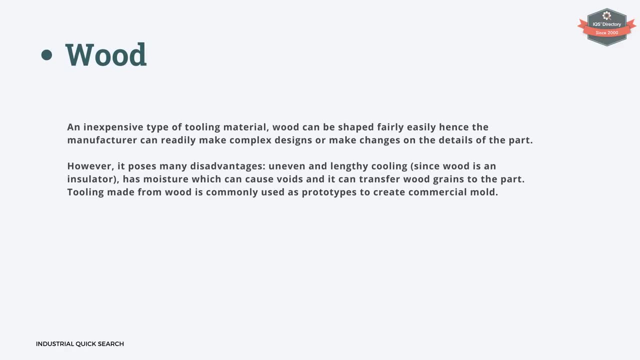 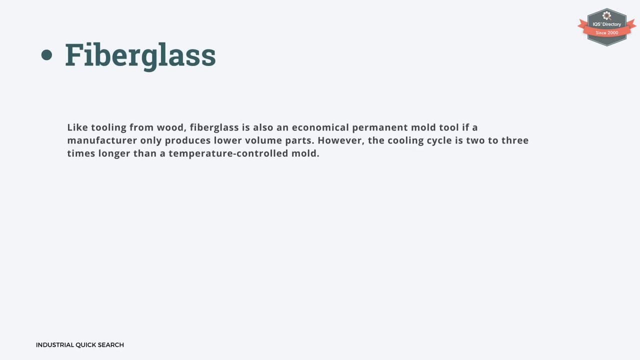 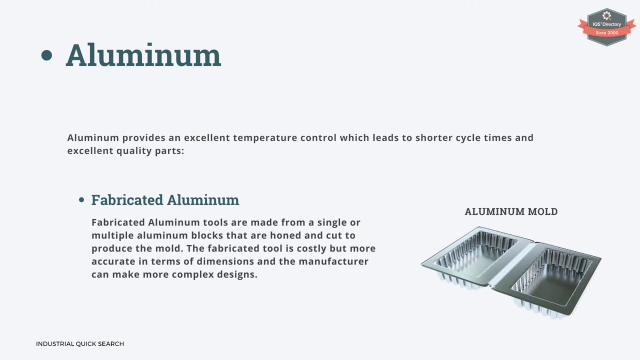 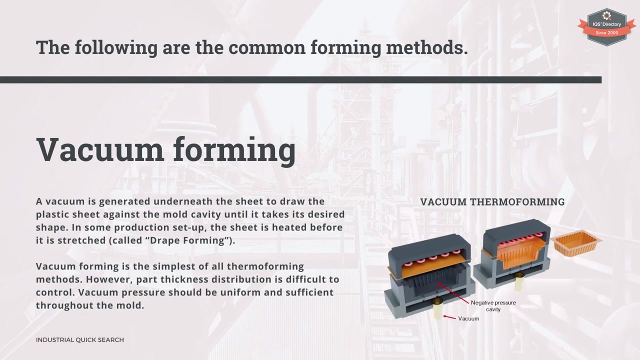 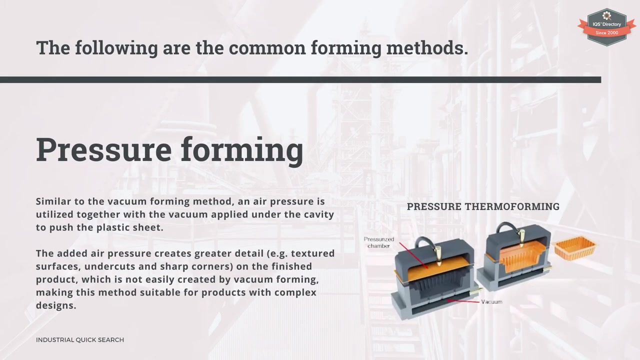 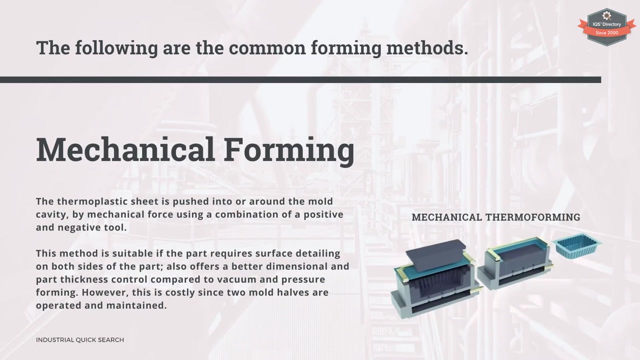 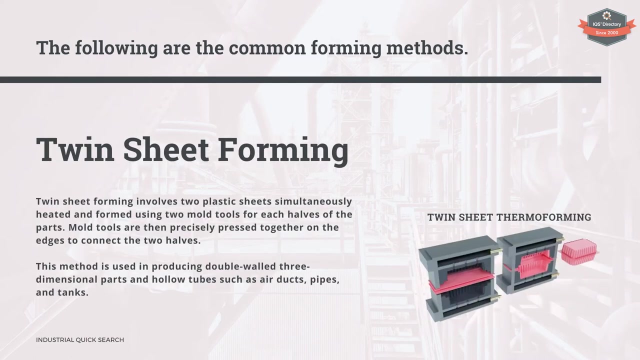 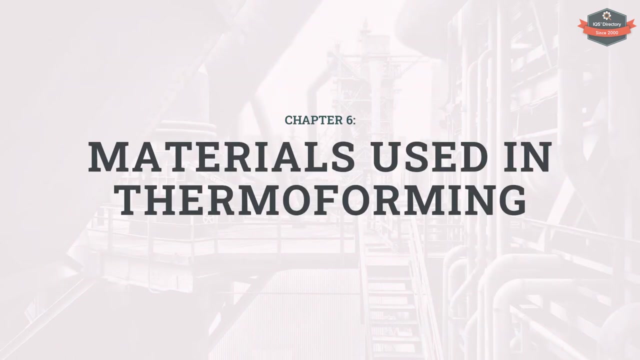 Chapter 3. Thick heavy gauge and thin gauge. thermoforming. Chapter 4. Types of molds. Chapter 4. Types of molds. Chapter 5. Thermoforming methods. Chapter 6. Materials used in thermoforming. Chapter 7. Materials used in thermoforming. 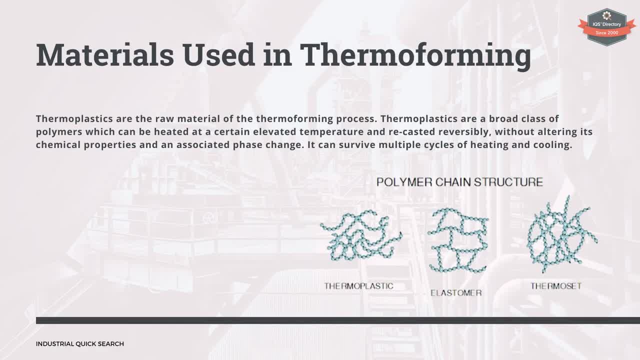 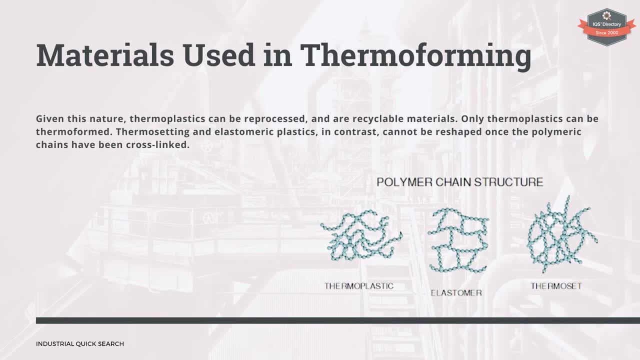 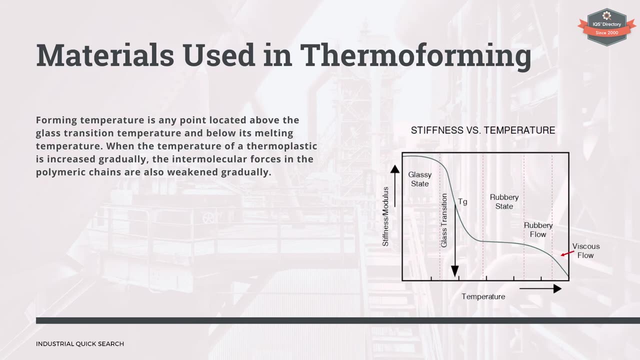 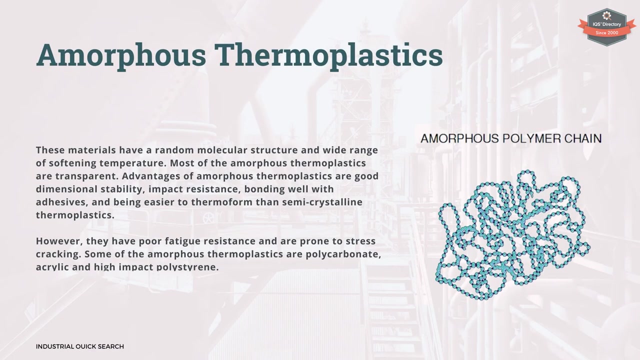 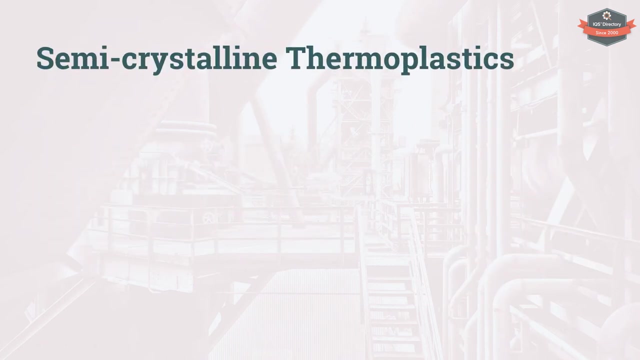 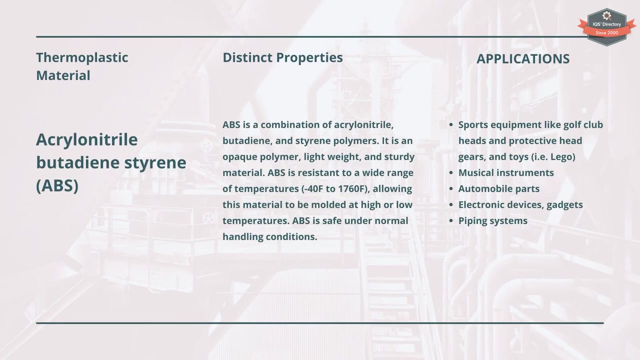 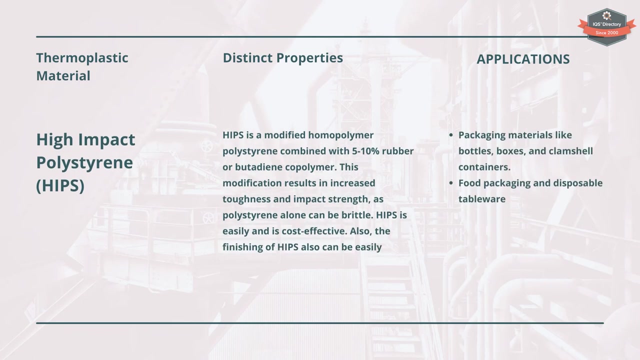 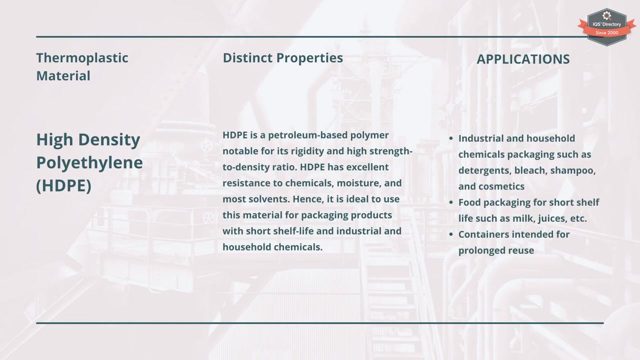 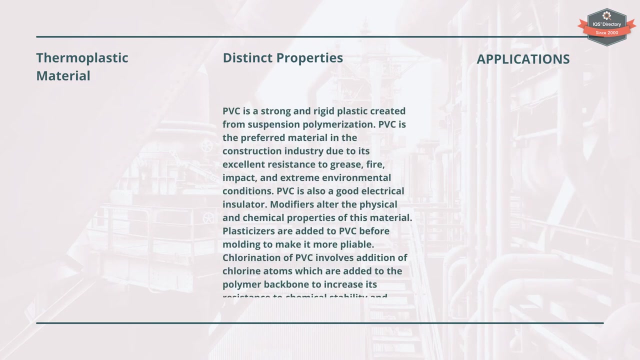 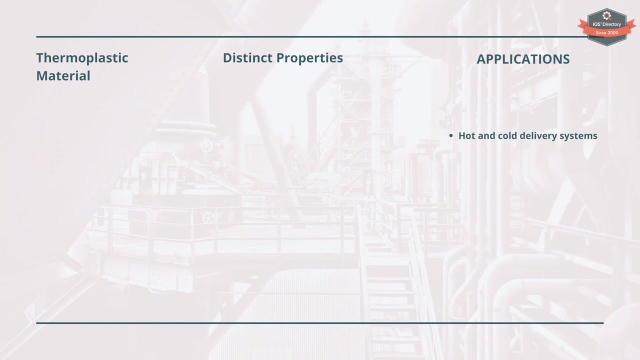 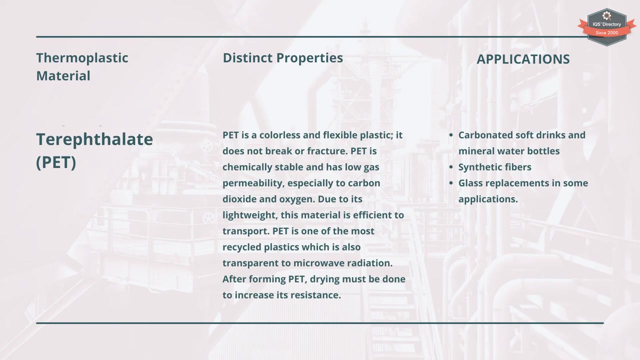 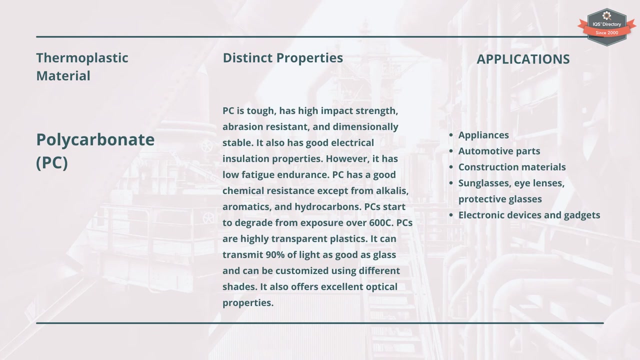 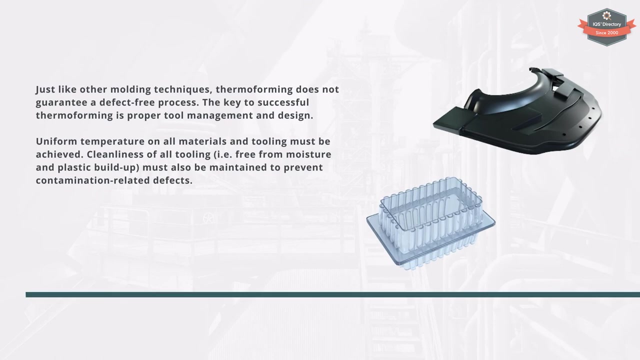 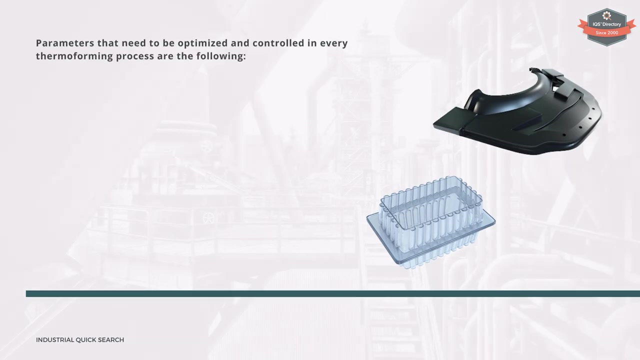 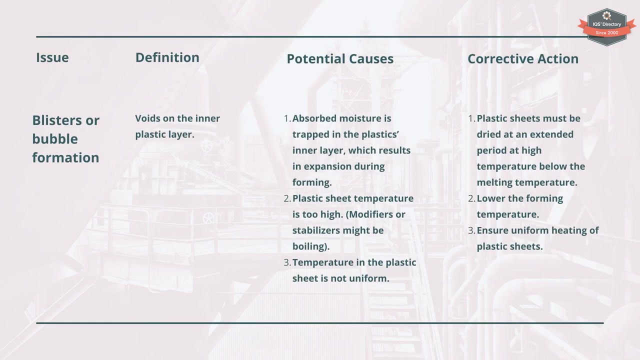 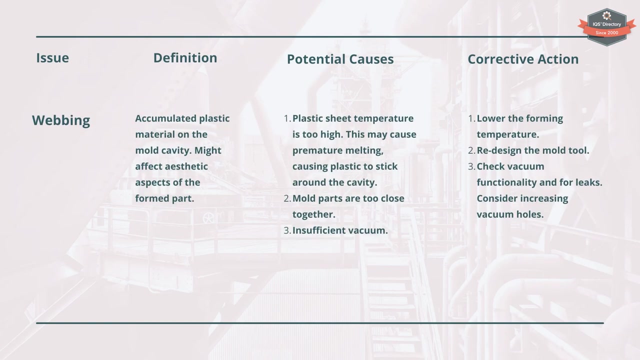 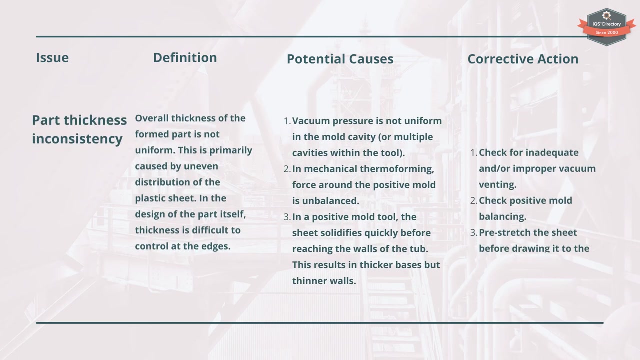 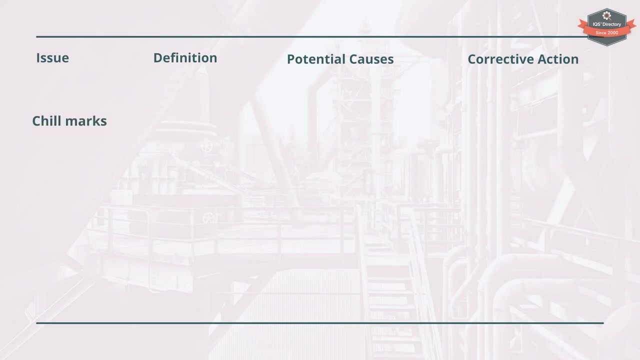 Chapter 8. Materials used in thermoforming. Chapter 9. Materials used in thermoforming. Chapter 10. Materials used in thermoforming. Chapter 11. Materials used in thermoforming. Chapter 12. Materials used in thermoforming. Chapter 13. Materials used in thermoforming. 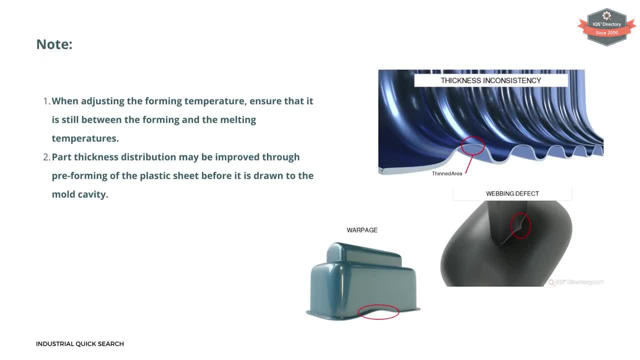 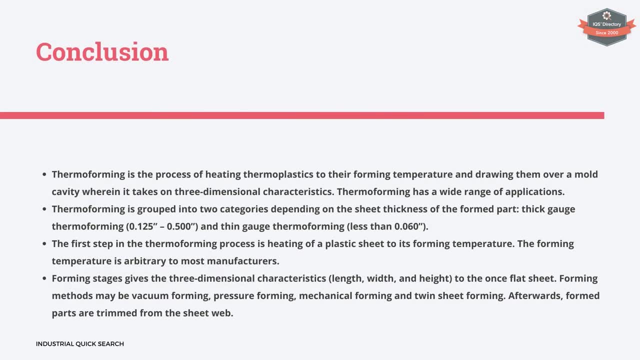 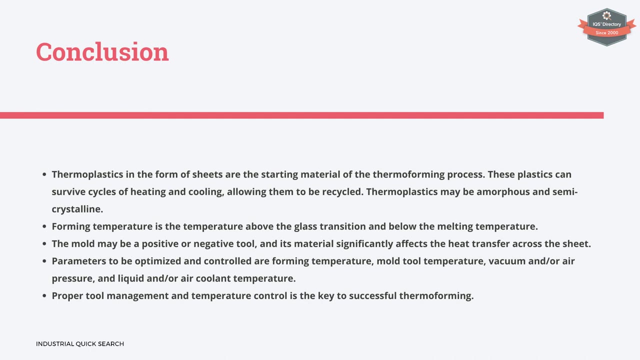 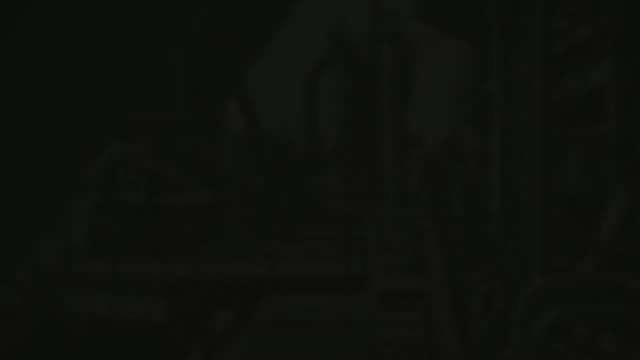 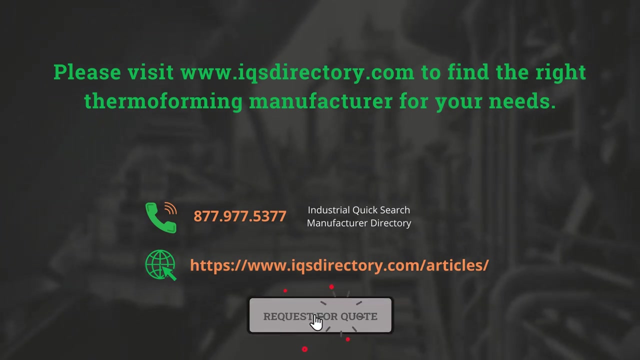 Chapter 14. Materials used in thermoforming. Chapter 15. Materials used in thermoforming.